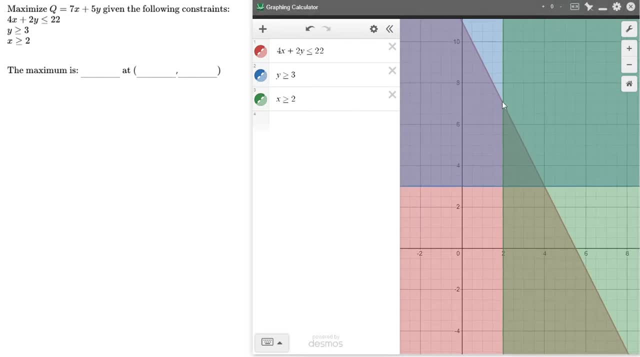 Where do they overlap? Okay, All of these inequalities- And I hope you can see, it's this little triangle right here. So that's what I'm interested in. The values I'm going to test now are all of the intersections. So right here. 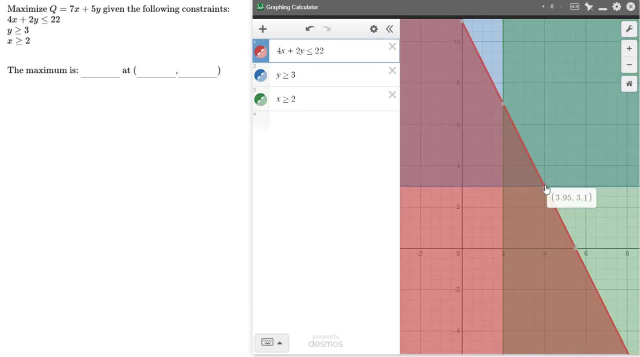 There's a point: 2, 7, 2, 3, and then 4, 3, right here. So again, where these three regions overlap, the intersections of those, are the values that are going to possibly maximize or minimize. 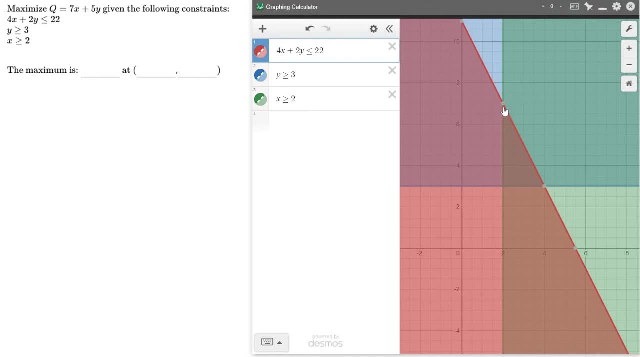 Now I can't just take the highest one and say, oh, that's the biggest one, It's going to maximize. That's not the case. You need to plug them in and test. So let's make note of those values and then we're going to test them. 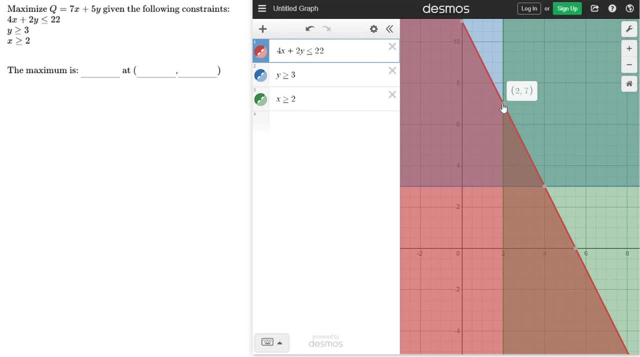 So 2, 7,. let me just write those over here, if I can find my cursor. So we've got the points 2, 7, and I think we also had 2, 3, right, So let me just make note of these. 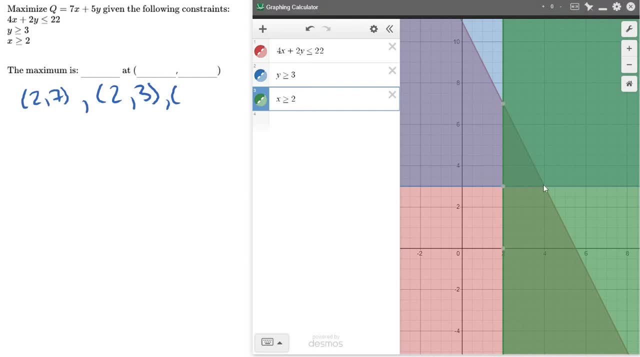 So 2, 3, and then our last one was 4, 3.. And depending on the equations they give us, you might have more points. You might have more points than you need to test. It just kind of depends. 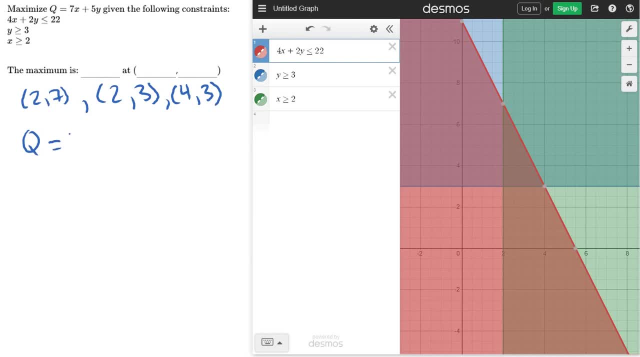 OK, now here's the big equation: Q equals 7x plus 5y. We just need to test each of these values, So let's go ahead and do that. So for this first point, I'd have 7 times 2 plus 5 times 7, right. 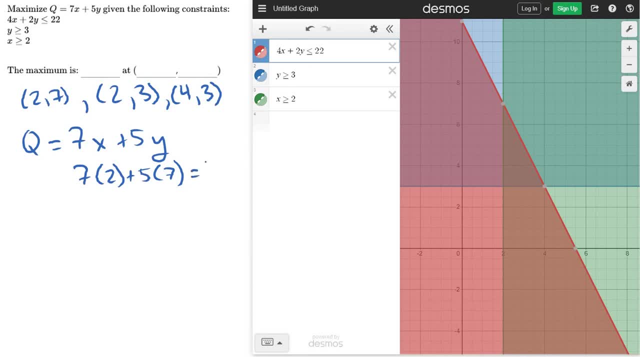 And so I get 14 plus 35. So 49 for that one. For the second one, I've got 7 times 2 plus 5 times 3.. This one's going to be smaller, but 14 plus 15.. 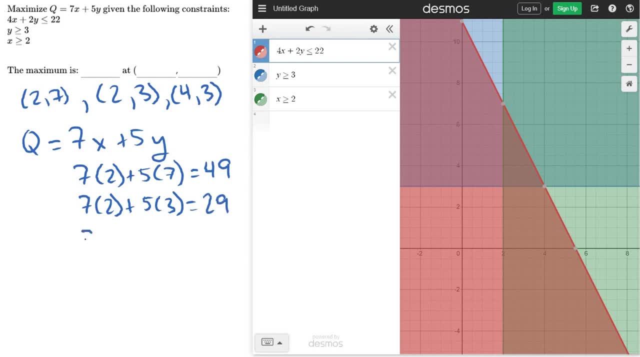 So that's 29.. And then for the last one I've got 7 times 4 plus 5 times 3 again, So I have 28 plus 15.. 28 plus 15, what's that? 43..